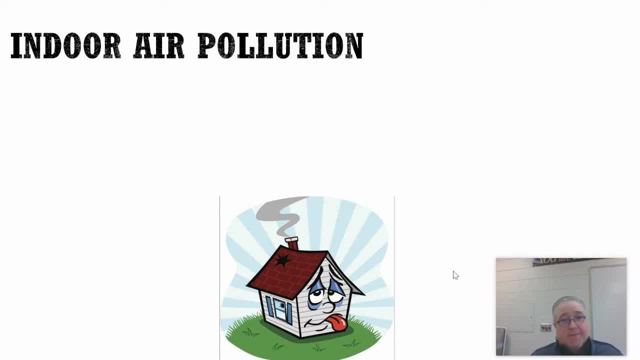 You know things like photochemical smog, for example, is a type of outdoor air pollution. So we're going to focus in this lesson about the indoor types of air pollution, And what's kind of interesting about indoor air pollution is it actually causes more deaths every single year compared to outdoor. 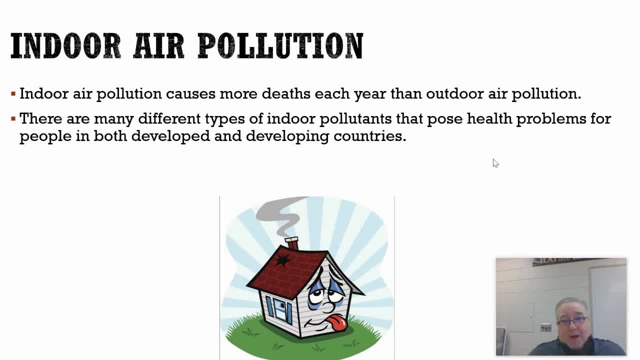 You know so, for all that stuff we talked about outdoor air pollution- how bad it was. more people die every year from exposure to indoor pollutants As compared to outdoor pollutants. Now, indoor air pollution kind of varies depending on where you live in the world. 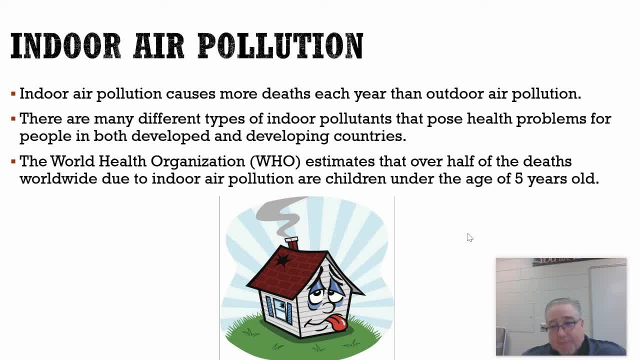 In developing countries, for example. you know the type of air pollution- indoor air pollution that they're exposed to is usually a little bit different from the indoor air pollution that the developed world is exposed to. So we'll kind of talk about both of those, reference both of those. 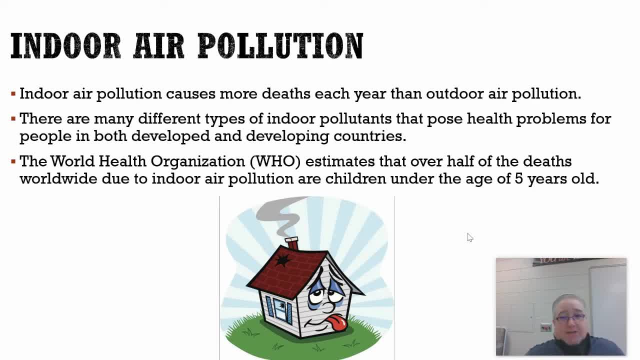 The World Health Organization, the WHO, estimates that over half of the deaths worldwide due to indoor air pollution are children under the age of five. So you know, a lot of these people that die are young children due to breathing in poor quality air. 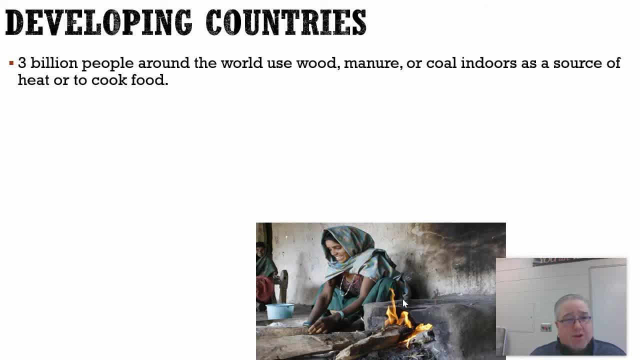 All right, so let's first talk about developing countries. We've kind of mentioned this a little bit before, About just some of the activities that take place inside the home In developing countries. So if you look at this picture here, for example, this woman is, you know, she has like a little fire pit, you know, either right outside of her house or possibly inside of the house, but you know in that she's burning wood or manure or maybe charcoal or something you know basically used to heat or to cook food. 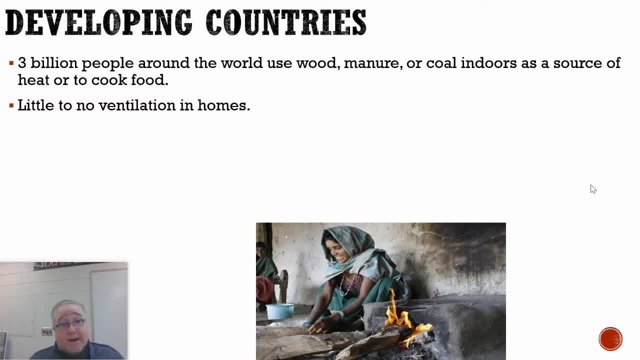 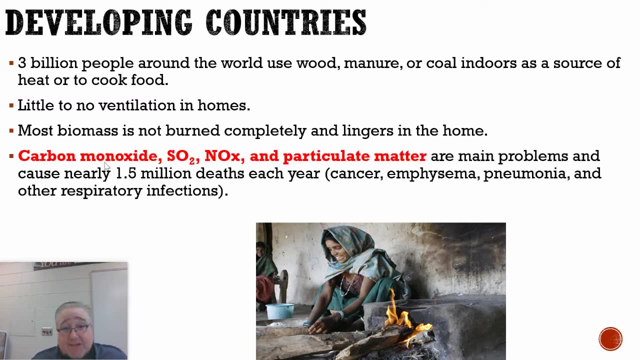 You know, a lot of these homes in developing countries have very poor ventilation. So that means a lot of these compounds that are produced, You know, from burning all this biomass just stay in the house and people end up breathing them in. You know things like carbon monoxide gas, SO2, NOx, particulate matter- these are all things that eventually lead to 1.5 million deaths every single year. 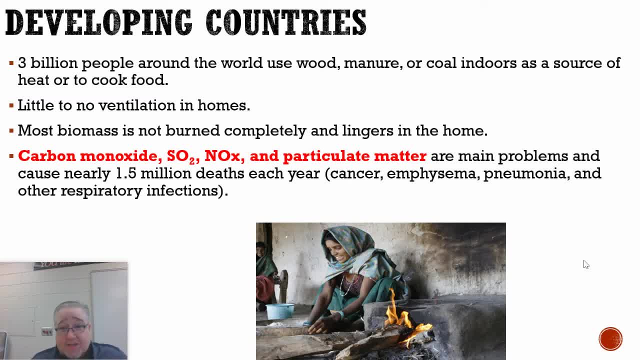 You know, mainly due to lung related diseases like cancer, emphysema, those types of things. So if you're burning a bunch of biomass in your house, it's probably not good for your health, But in developing countries this is the only access they have to a fuel source so that they can cook their food. 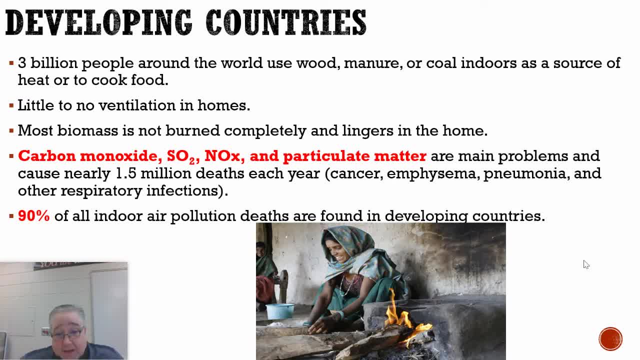 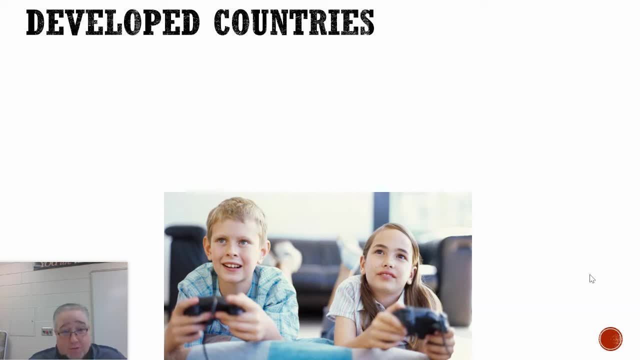 Not everybody in the developing world has natural gas and electricity, So this is what they're going to have to use. 90% of all air pollution deaths are found in developing countries, So remember that statistic. Now, as far as the developed world goes, you know, you know, like the United States. 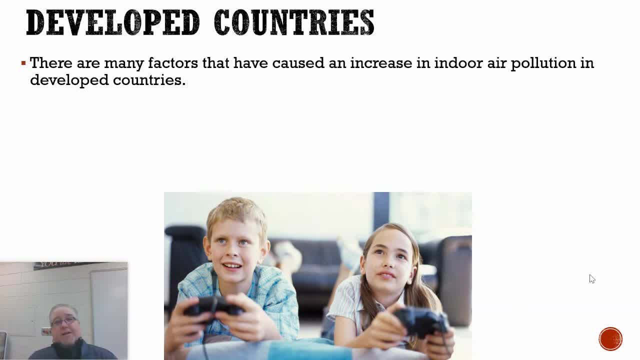 For example, you know, there's a few factors that kind of come into play that help increase the amount of air pollutants inside the home. You know, one of the things that we're seeing is that in the developed world indoor air pollution exposure is increasing, partially because people are just spending more time indoors. 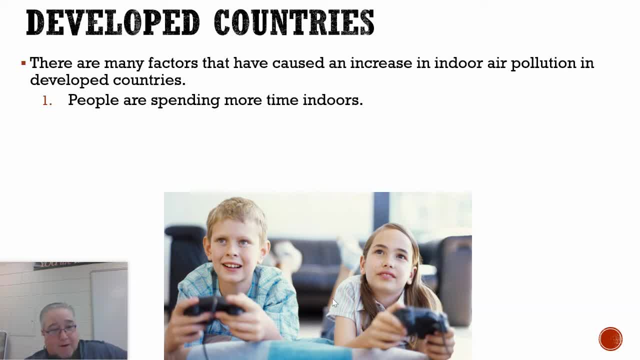 I mean look at these two kids right, They're inside playing video games For probably five, six hours at a time. you know, go outside kids. I mean get out of your house. I mean the more time you spend inside the house, the more time you're going to be exposed to indoor air pollutants, if there are any. 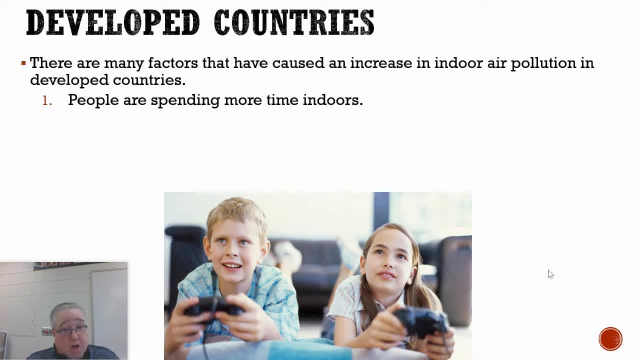 And there usually are some inside of everybody's home. We'll talk about some of those things in a minute. Our homes are much better insulated than what they ever used to be, So the better insulation you have in your home, the more that air is going to stay inside your house for a longer period of time. 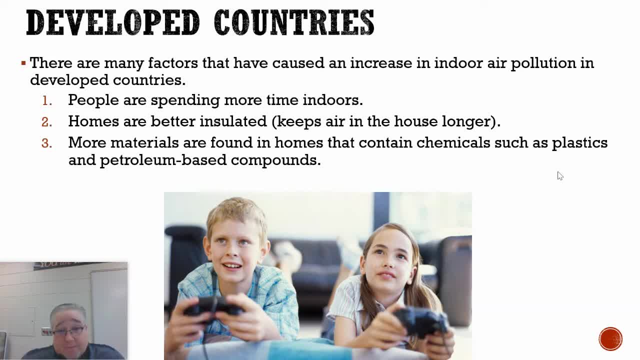 And again, you know, there's more materials in the home, now more than ever, that contain chemicals that could end up being indoor air pollutants, Things like petroleum-based compounds, plastics- We talk about box compounds. Again- these are all things that we don't want those odors to be inside the house. 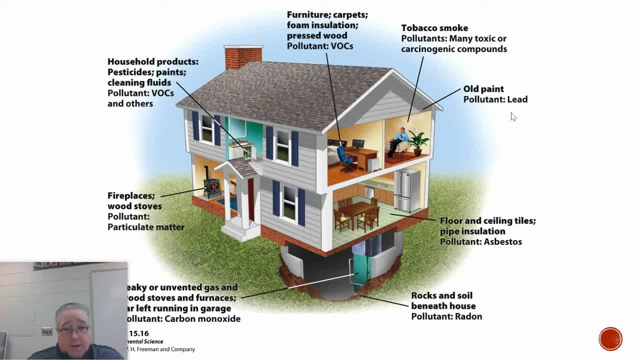 Here's just some examples- and you can read this on your own- of some different indoor Indoor air pollutants. You know, it could be something as simple as tobacco smoke. if anybody in your house is a smoker, It could be old paint. You know, it could be asbestos. We'll talk about that in a little while. Radon gas: particulates from fireplaces or wood-burning stoves. 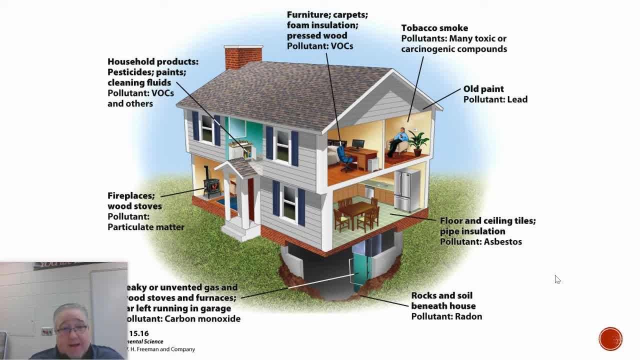 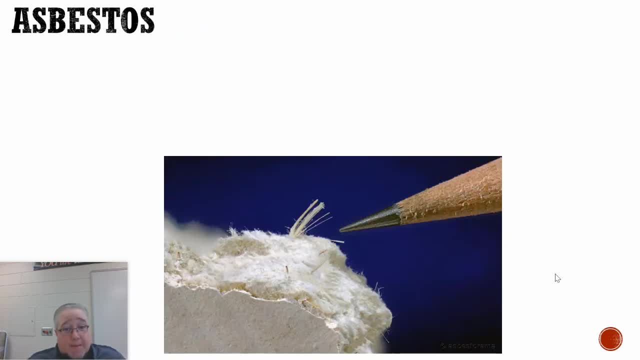 And again, a whole bunch of chemicals as well that can linger inside the house. So these are all things that you know. chances are we have at least one of those things in our home. I want to talk about a couple of specific types of indoor air pollutants. 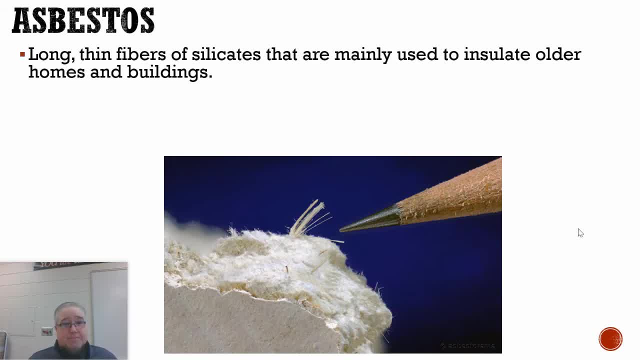 One of them is called asbestos. Asbestos is a material that used to be used as an insulating material in older homes and buildings. It's not used anymore, and mainly that's because of what it's made of. It's made of these thin fibers of silicate. 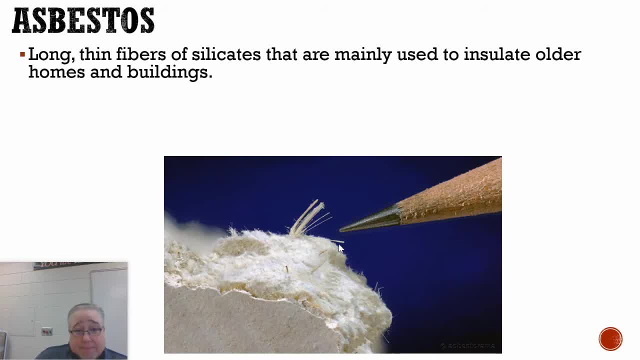 Silicate is basically glass And this, actually this material does make for a very good insulator of the home. You know they would insulate the inside of the walls and the ceilings, you know, with asbestos. But what they found out, this was back like in the 1970s. they found out that. you know this stuff, if it becomes airborne you can breathe it in. 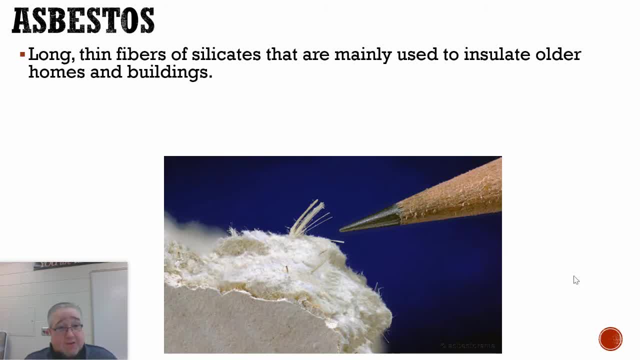 You can get extremely sick from it. So all the asbestos that was used, You know, in some of these older homes and buildings had to be removed. The thing is to remove it you have to be extremely careful. You don't want to just rip it out of there. 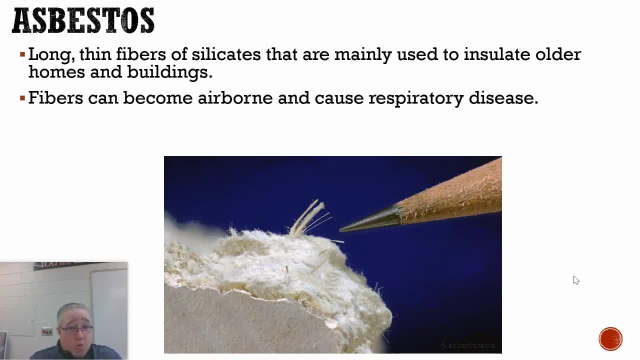 You have to take it out very carefully because if you rip into it and those particles become airborne you can get them in your lungs. That's called asbestosis And that can be very dangerous because it can lead to a type of lung cancer called mesothelioma. 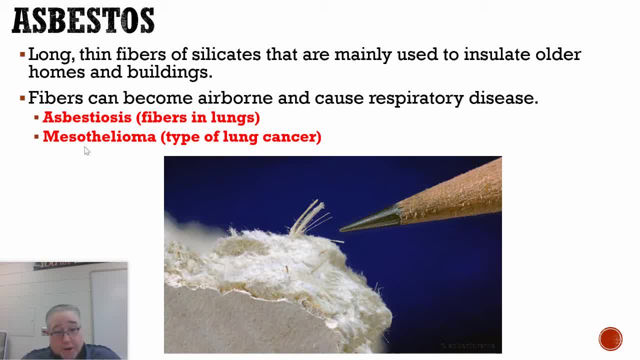 Maybe you've heard of that before. They have commercials for it. You know there's lawyers that specialize in mesothelioma cases, But asbestos, again, it's one of these things where you know modern day homes are not insulated with asbestos anymore. 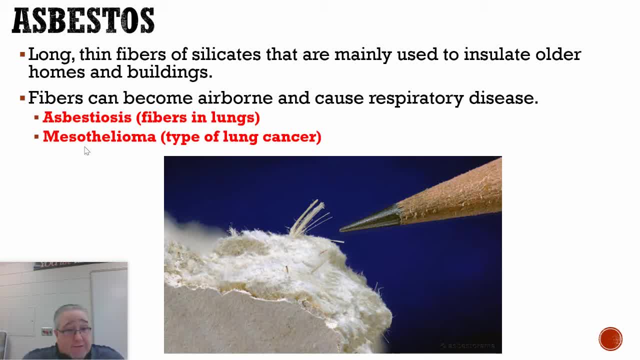 But you know older homes, maybe homes built back in the 1950s and 1960s. those homes, some of those places, may still have asbestos in them, especially if they're abandoned buildings and things like that. They may still have those fibers there. 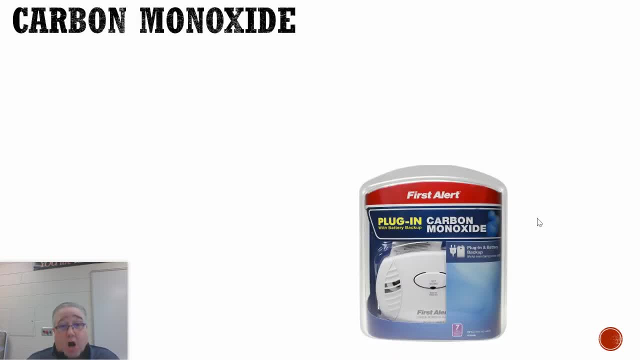 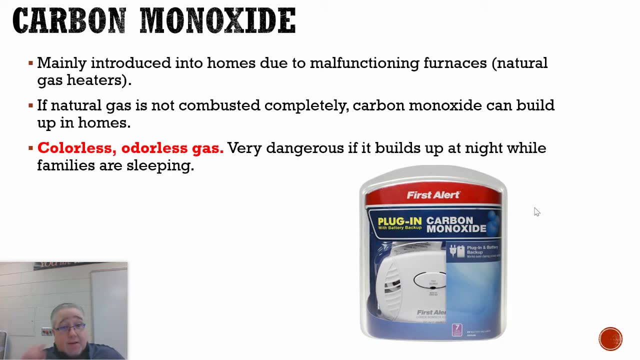 So you have to be very, very careful with that type of thing. Carbon monoxide: This is another indoor air pollutant. This usually is released due to a malfunctioning furnace in your home. It's always a good idea to have your furnaces inspected, maybe on a yearly basis or, at the latest, maybe every other year. 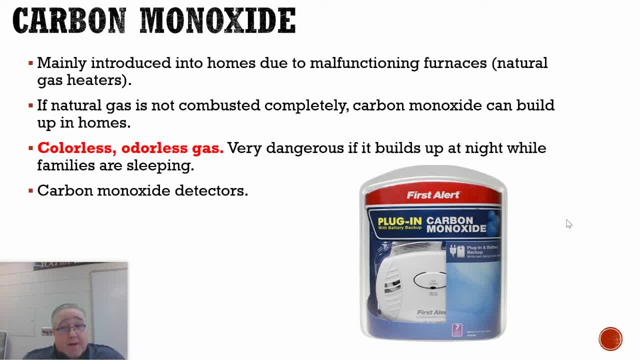 Because if those furnaces are malfunctioning, they may not be burning the night, They may not be burning the natural gas the way that they should be, And that carbon monoxide can actually be released inside the home. The carbon monoxide is a byproduct of incomplete combustion of natural gas. 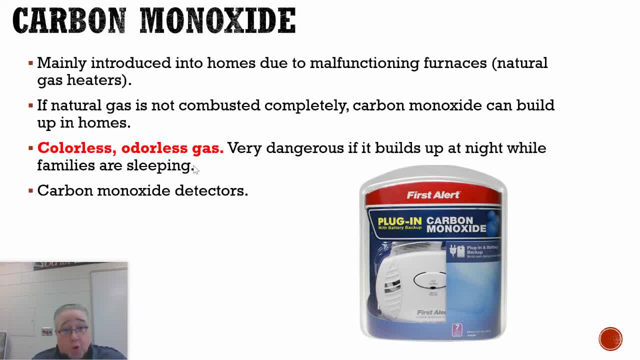 So if that builds up inside the home again, it's a colorless, odorless gas- We've talked about that before- And if you breathe it in you get very sick. You know, if it's nighttime and you're sleeping and you breathe that in, you may not wake up. 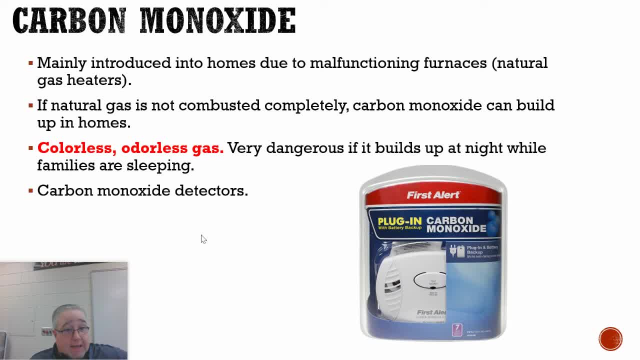 There are people out there. They may not wake up. There are people who die in their sleep from breathing in carbon monoxide fumes. They do sell carbon monoxide detectors, You know. I highly suggest that every everybody's home has at least one of those installed, just in case there is a carbon monoxide leak or some type of carbon monoxide buildup inside your house. 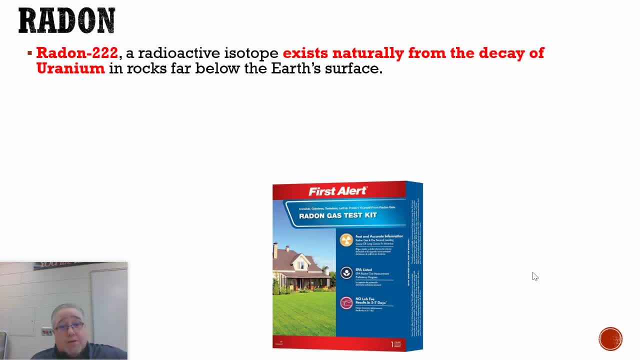 Radon is another indoor air pollutant. Radon gas typically is caused by Radioactive decay of uranium that is below the surface of the earth. There's uranium in the earth that's deep within the earth's crust, But it's a naturally radioactive element. 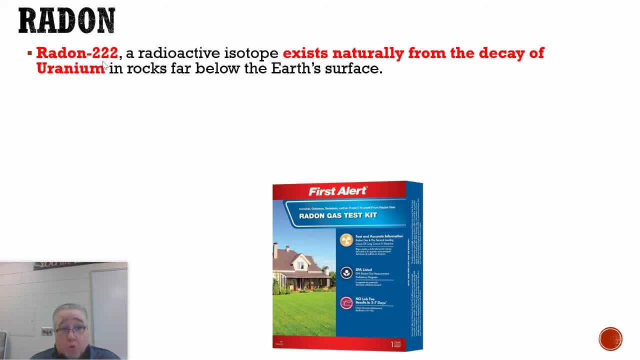 And when it does break down, it produces radon 222.. Radon is a gas that will seep up through the surface of the earth, And if there's any cracks in the surface, then it can enter your home. You can even get into groundwater as well and seep into the house through a well. 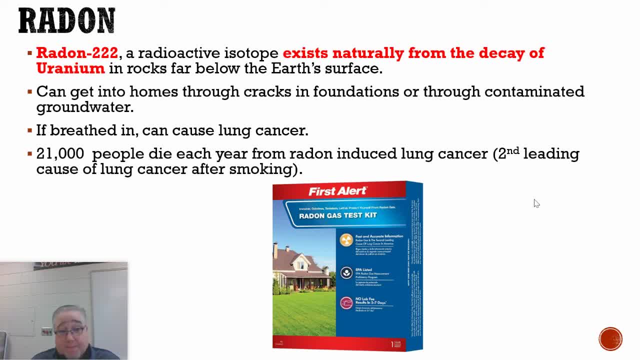 And if you breathe it in it can definitely cause problems. In fact it says here: 21,000 people die every year from radon induced lung cancer. It is the second leading cause of lung cancer after smoking. So I mean radon gas is a real deal. 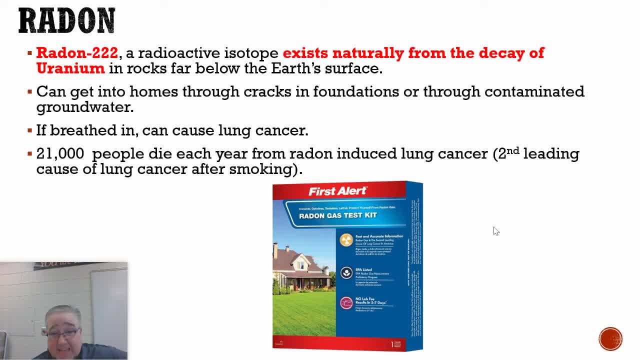 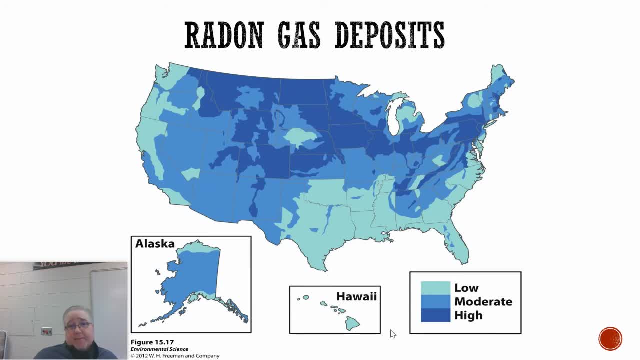 So again, there are radon gas kits that you can purchase. I have those in stock, I have those installed in your home. You know, this is a map showing us just some of the common radon gas deposits around the country. 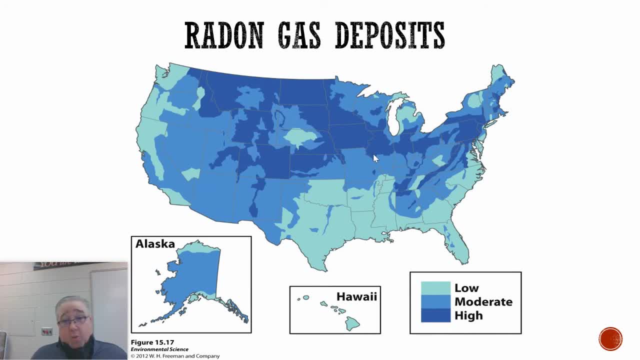 And you will notice. you know right up here where we live, you know right up in northwest Indiana there is a very high amount of radon gas underneath the surface. So you know, if you have an older home especially, and there's a possible crack in the foundation of your home- you know underneath the house- then some of that radon gas could leak in. 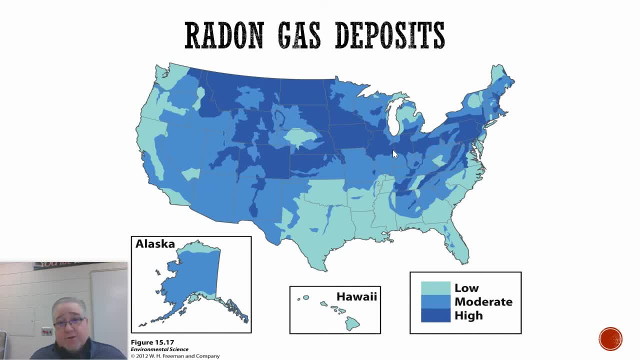 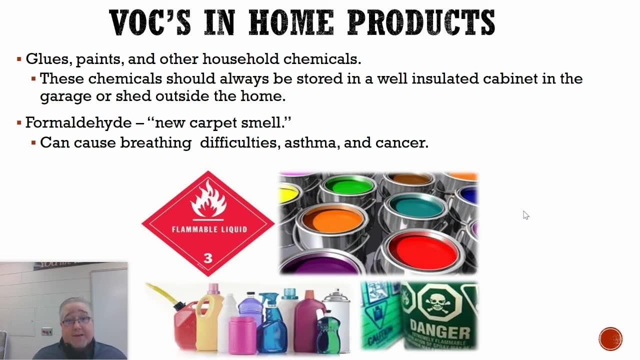 So it's a really good idea to have that inspected. Have those radon detectors in your home to make sure that that does not cause an issue. VOX compounds: we've talked about these. These are things also that are found in the house. 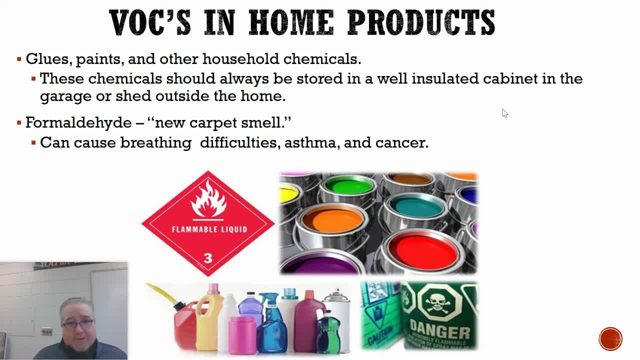 Things like paints and glues, And we talked about air fresheners, things like that. You know these things especially. you know paints and things that have a strong odor to them. you know those things should always be stored, you know, in a cabinet, you know inside of your home. 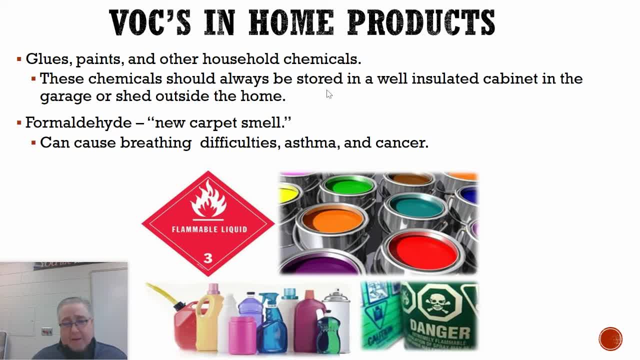 Right Right In your garage or even, if possible, in a shed that's far away from your home. That way those fumes won't build up inside the house. Formaldehyde, that's what produces the new carpet smell. So if you get new carpeting installed in your house, you know that could cause difficulties breathing, could cause asthma, could even cause cancer. 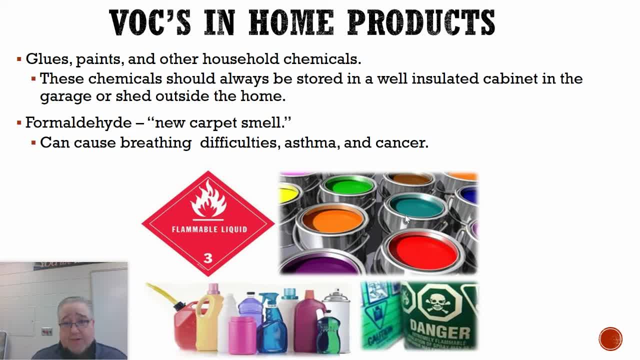 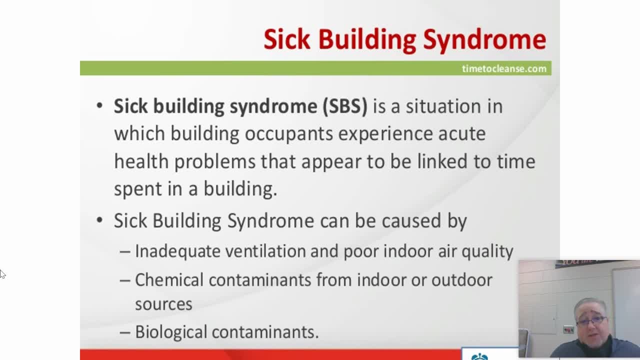 Luckily, that smell does dissipate after a while, So that's kind of a good thing. And then finally, today we have something called sick building syndrome. Sick building syndrome is a situation where people who are working, let's say, for example, in an office building- people get sick due to the conditions of the building itself. 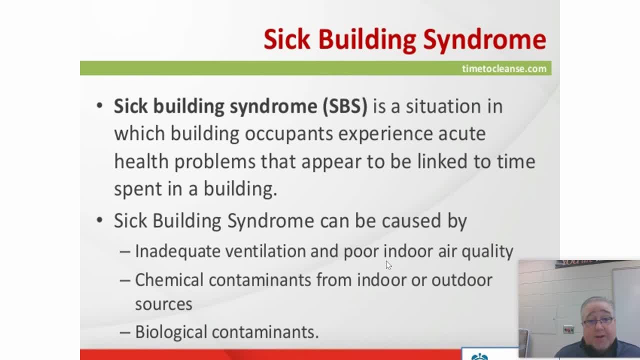 Sometimes there's just inadequate ventilation in the building. Sometimes there's chemical contaminants from an indoor or maybe even an outdoor source. Sometimes there's biological contaminants. There's things like mold, for example. We see sick building syndrome. you know, usually in older buildings that may be susceptible to mold.